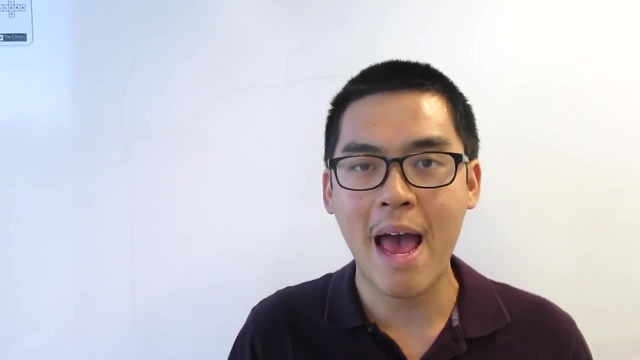 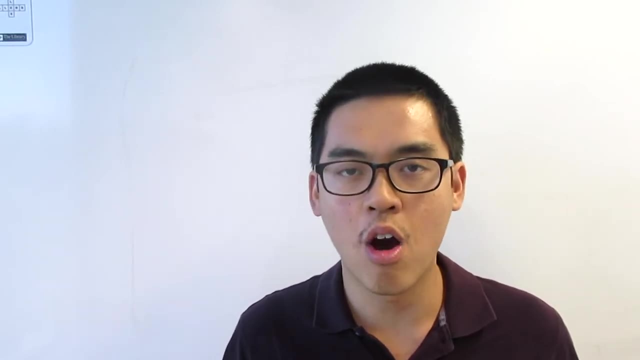 in your closet and then you want to pick three of them to put in your bag so you can go on a weekend trip. So, for simplicity, let's call those shirts that you have in your bag n-choose-k: Shirt one, shirt two, shirt three, all the way to shirt seven. And what are some ways to pick? 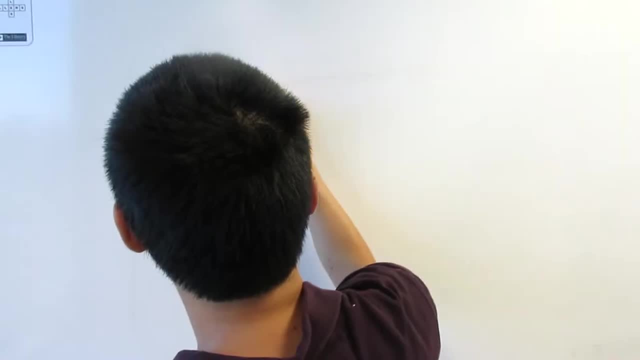 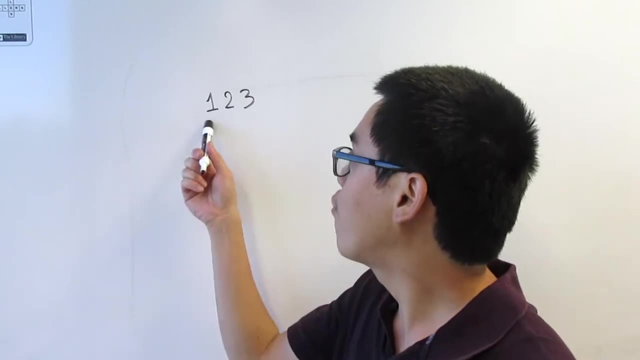 three shirts. Well, you can do one, two, three, All right. And one important thing about n-choose-k thingy is we don't care about the order. So once you have one, two, three, you don't consider one. 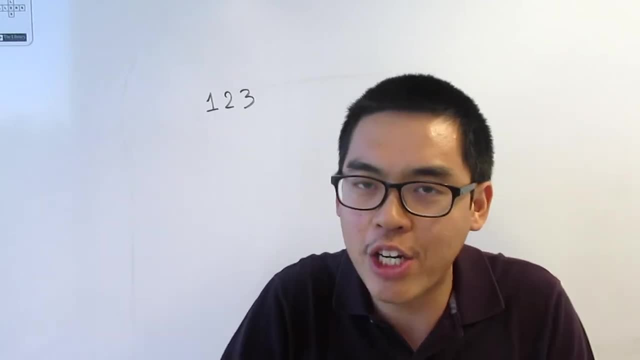 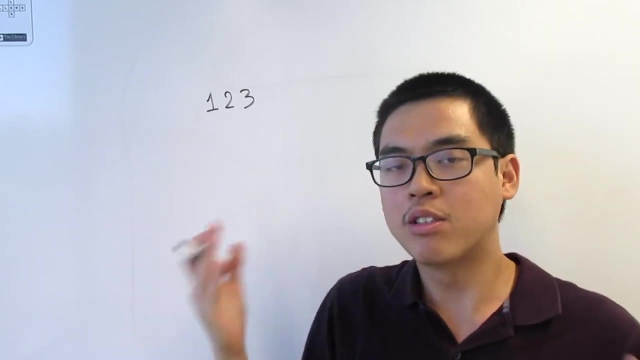 three, two as different configuration, because you just put three shirts in your bag, right? It doesn't matter which one you put in first, You're going to pack all of them there anyway. So one, two, three will be considered the same as one, three, two. 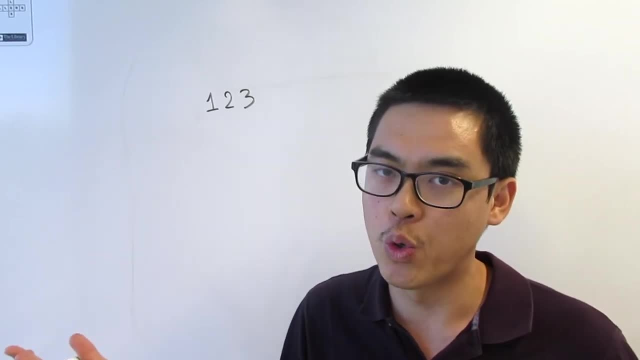 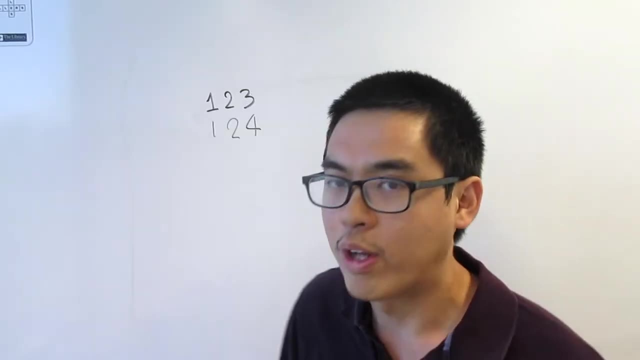 So if you want to list all possible way out, you don't list one, three, two as another combination. So we have one, two, three here. What's some other way? Well, we can do one, two, four, one two, five, one, two, six, so on and so forth. 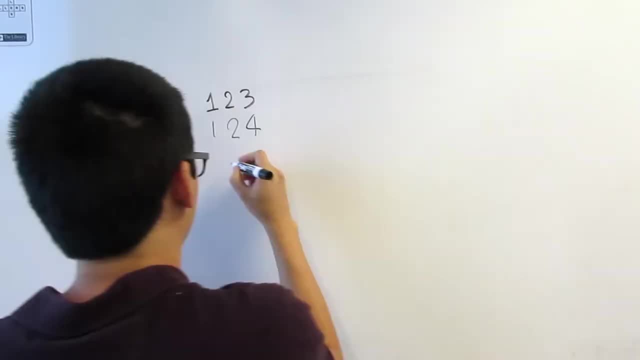 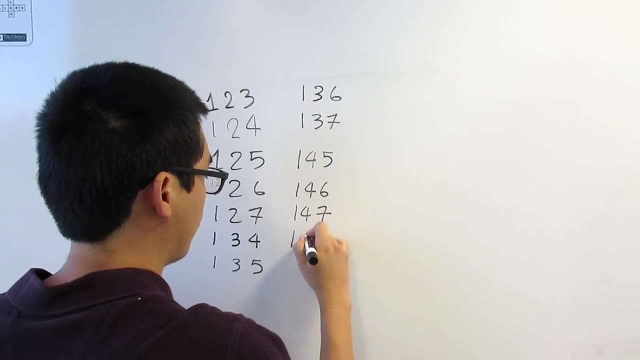 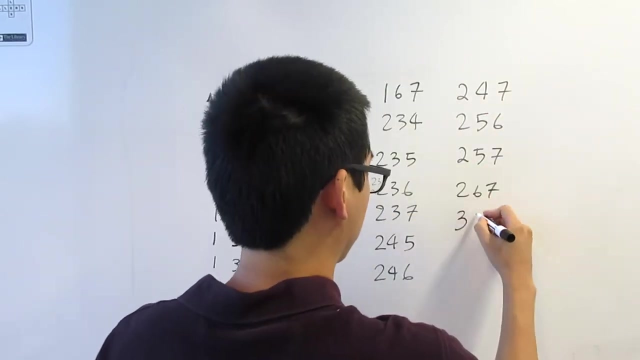 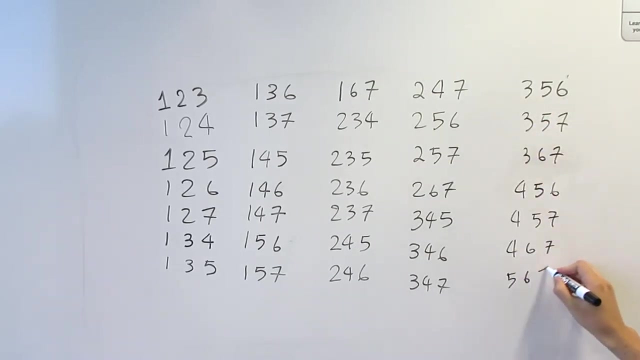 So in this case, let me actually list everything out for you All right, Here they are. I think I have them all. So if you just come up with three random number between one to seven, you should find your sequence there, Like if you've one, two. 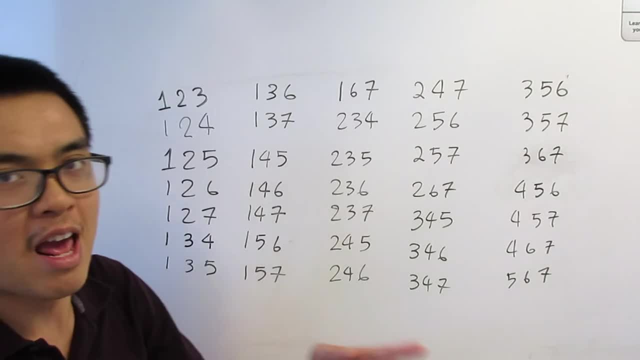 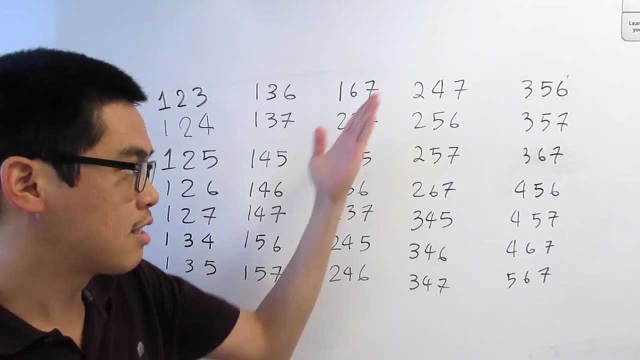 four and seven. two four and seven is right here, right, And if you come up with any random number, it should be one of these combinations. So seven choose three is the number of configuration we have on this board. So let's count how many are there? 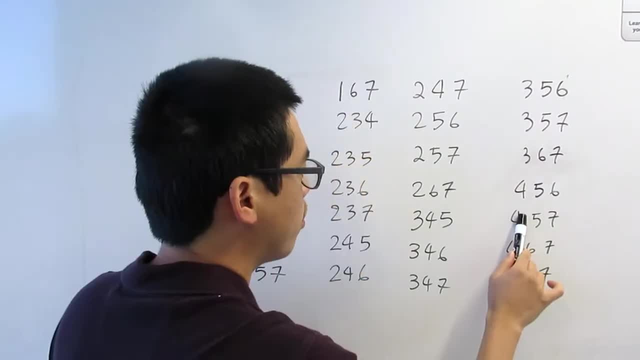 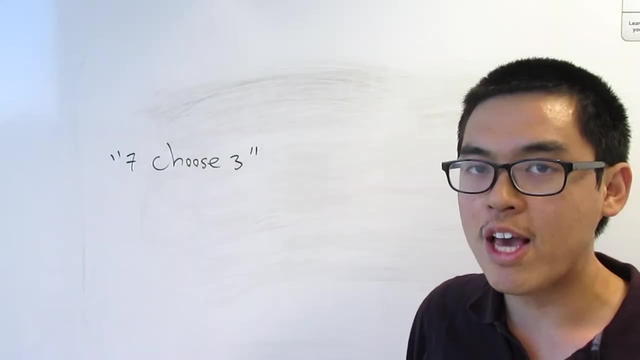 One, two, three, four, 15,, 16,, 17,, 33,, 34,, 35.. So seven choose three is 35.. All right, Notation wise, we're going to write seven choose three as something like this: 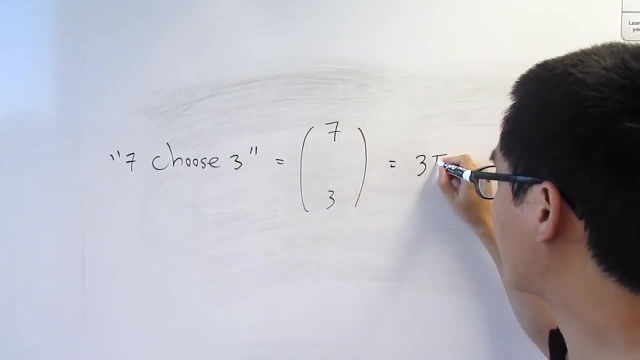 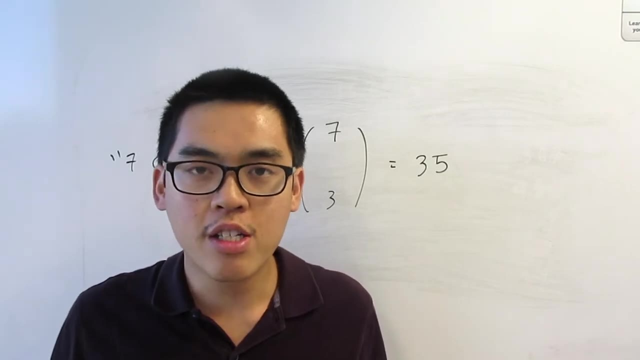 Seven choose three is 35, because there are 35 ways to pick three numbers out of seven. All right, And if you're adventurous you can try to compute eight, choose three. eight choose four, 10, choose five by yourself. It's going to be very tedious to compute those. 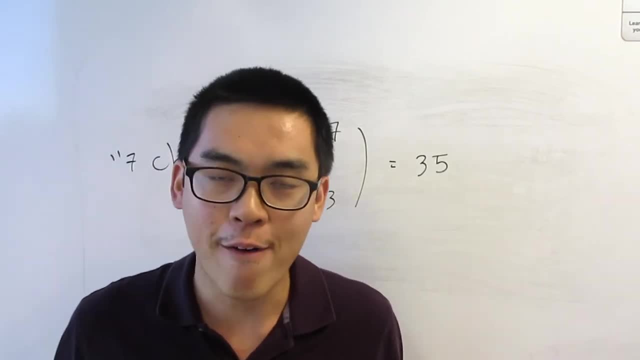 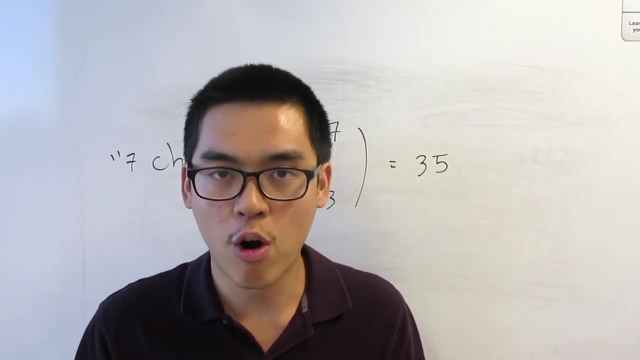 number. if you want to do it the way that I did- And that's why we have formula In order to know how many ways to do those configuration, instead of listing them all out, you can just use the following formula to compute and choose K. But before I go over formula for and choose, 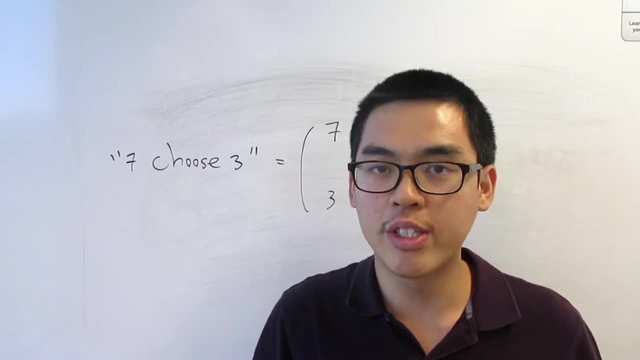 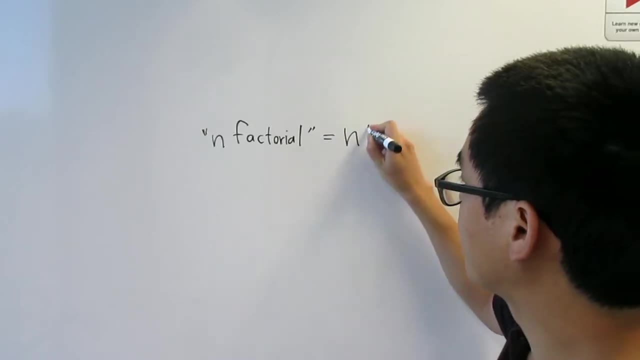 K. I need to introduce another formula really quickly first, which is formula for factorial. All right, So N. factorial, which is denoted by N with exclamation point, is another combinatorial number, which means this number count, the number of ways to do something, And in this, 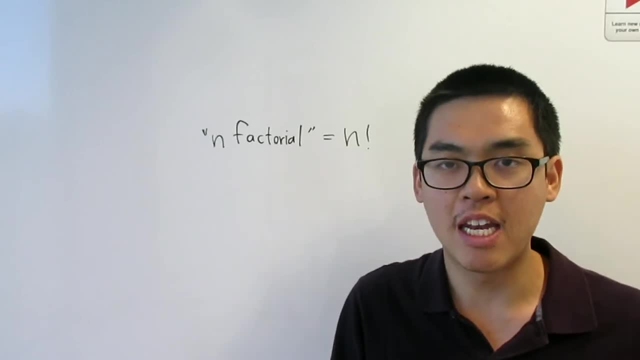 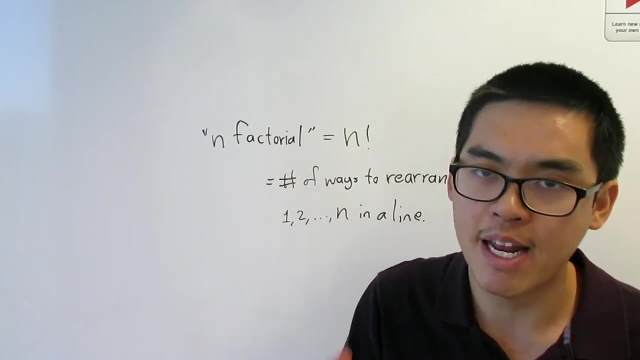 case N factorial, count the number of ways to rearrange N number in the line. All right. And formula for N factorial is: N factorial is the same as N times N minus one, times N minus two, all the way to two to one. 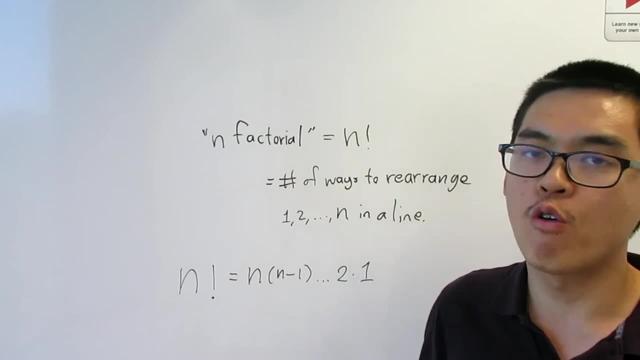 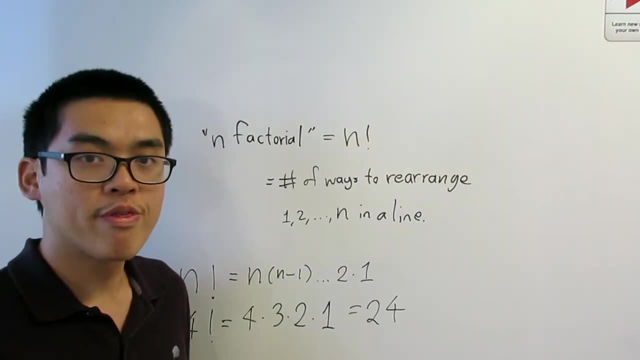 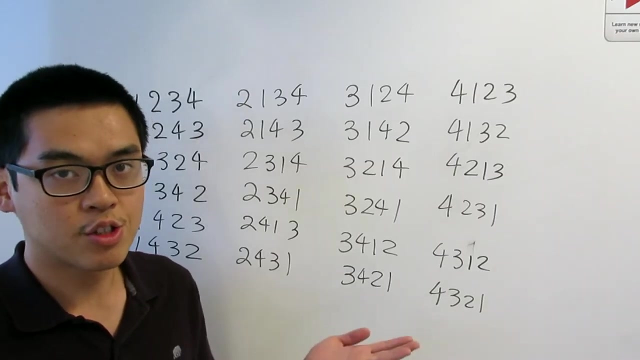 As an example, to compute four factorial. four factorial is just four times three times two times one, which gives you 24.. So with that there should be 24 ways to rearrange number from one to four. And here they are All right. So these are all the ways to rearrange four numbers. 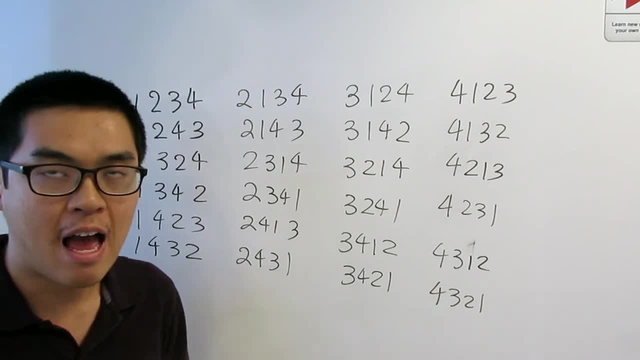 So if you have number one, two, three, four and you want to line them up in the line, maybe you want three first and then you want two, and then you want four, you want one- you end up with three, two, four, one. 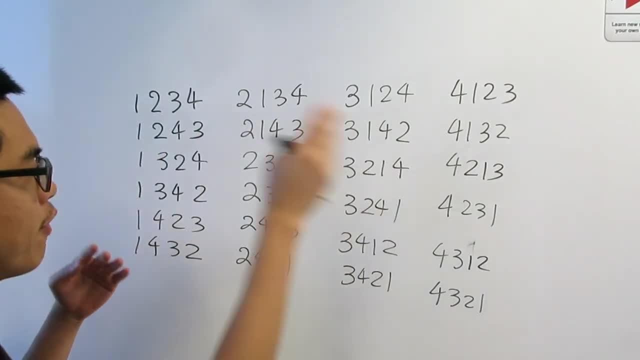 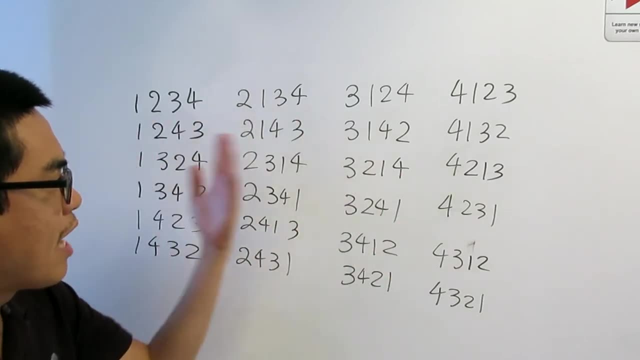 That configuration should appear on this board. So three, two, four, one is right here And anyway you want to rearrange. it should appear as one of this configuration, And there are 24 of them. All right with this, we are ready to dig into. the formula for N choose k, All right. So formula for N choose k low, we have N factorial on top, n minus k factorial on the bottom, and also n minus k factorial on the bottom, All right. So let's actually do one example before we compute seven quintuplets of. 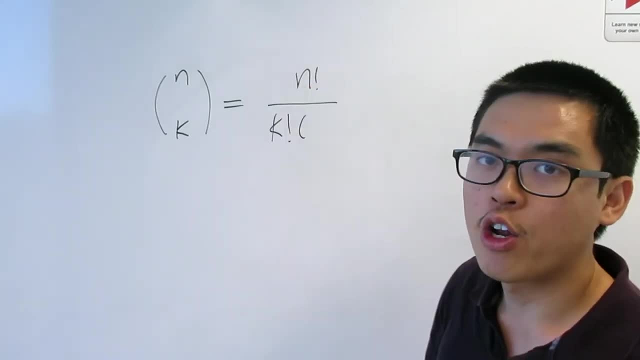 factorial. Now this s careful, So let's write: the expression of N is equal to, and n minus k factorial is the other formula, which is n minus k factorial. It is challenging to write n times k factorial, right? So let's actually do one example before And again. 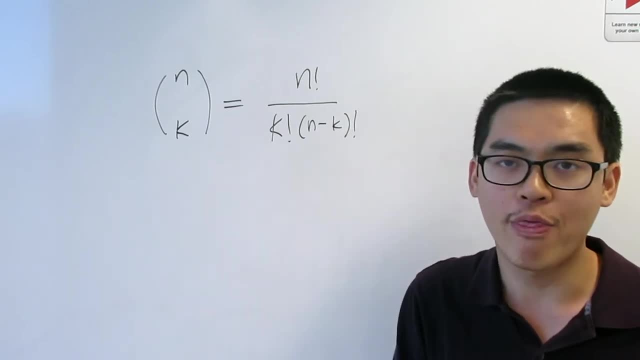 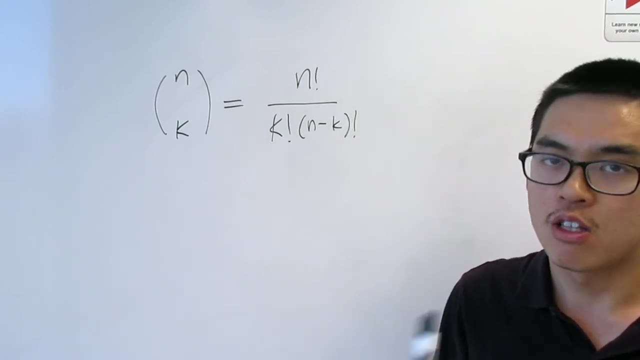 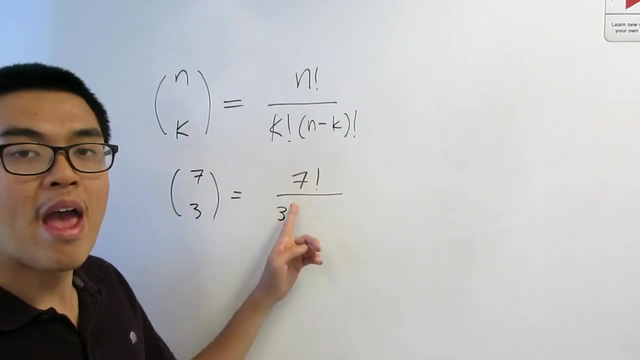 Before we compute 7 choose 3 right by, just list everything out and we get 35. So hopefully, if you pop n equal to 7, k equal to 3, use this formula, the result should be 35. Let's do that. So what is 7 choose 3? 7 choose 3? just 7, factorial on top, 3 factorial on the bottom and the way. 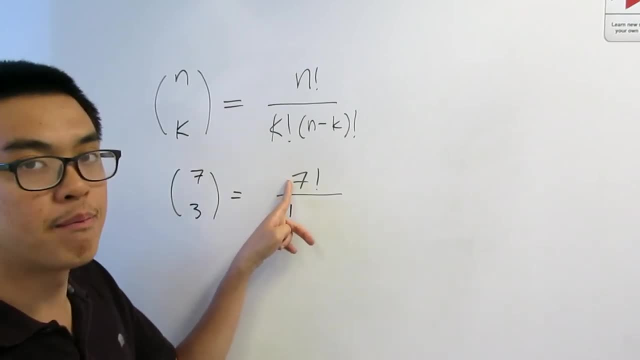 I memorize this is the other factorial. should add to this, become the top number. So we have 7 here. We have 3 here, So we have 4 left. So it's 4 factorial here. every time you compute n, choose k. Please don't multiply everything now and divide at the end because you want to do cancellation first. 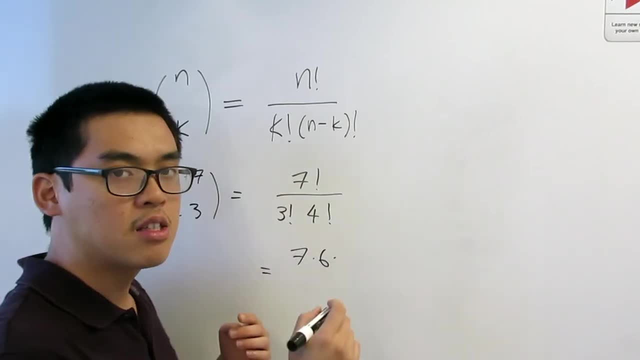 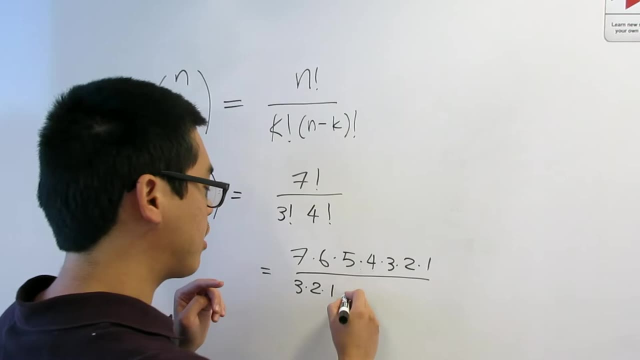 so let's pass 7 factorial out as 7 times 6, all the way to 1. 3 factorial gonna be 3 to 1. 4 factorial gonna be 4 times 3 times 2 times 1. All right, and don't multiply out, just yes. 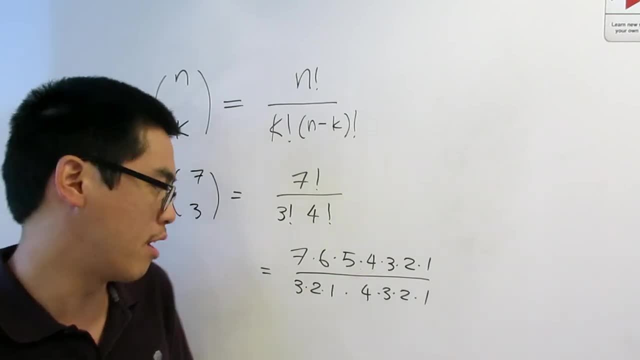 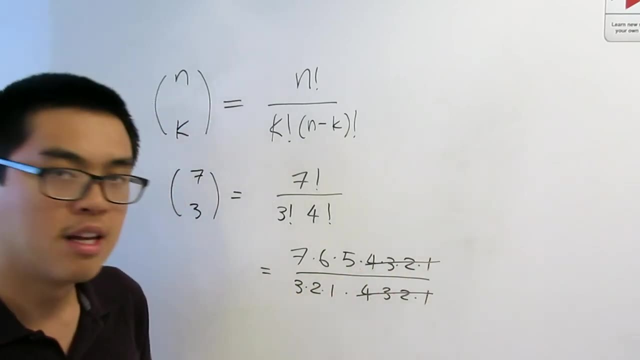 Try to do a lot of cancellation first and then multiply at the end. in this case, You see 4, 3, 2, 1 here, and also 4, 3, 2, 1. Yeah, so you can do cancellation like this, and Then you have 3 times 2 here and 6 here. So 3, 2 and 6, and 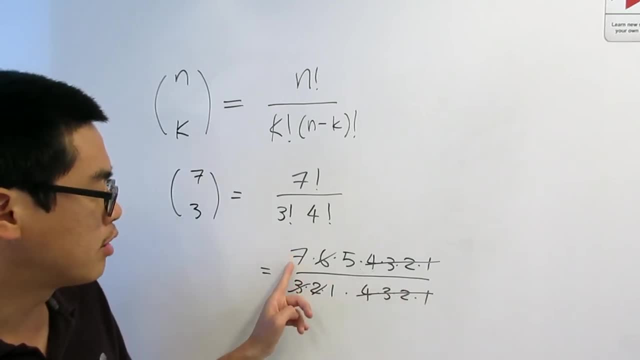 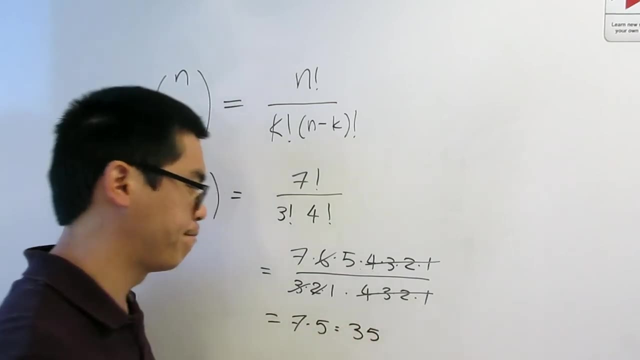 At the end all the bottom numbers are gone. at the top you have 7 and 5. So the answer is 7 times 5, Which is 35. So of course in choose k is helpful when you want to count the number of way to pick some number of objects. 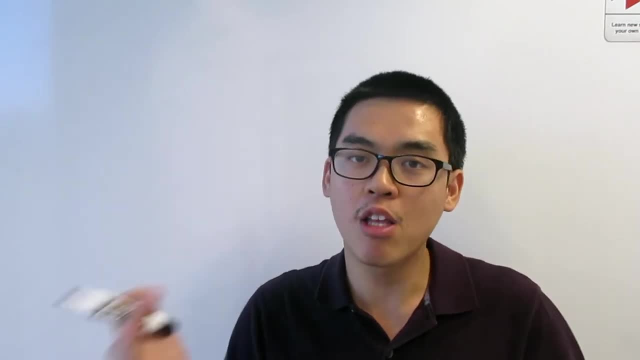 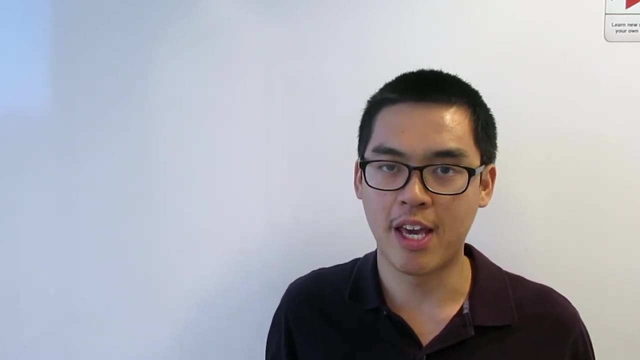 From the bigger set of object. but sometimes the problem is not phrase that way, But you can still use n, choose k to attack the problem, and, and these are a few problem that you can use in choose k. So let's go to those examples, So let's count the number of way to rearrange these seven letters. 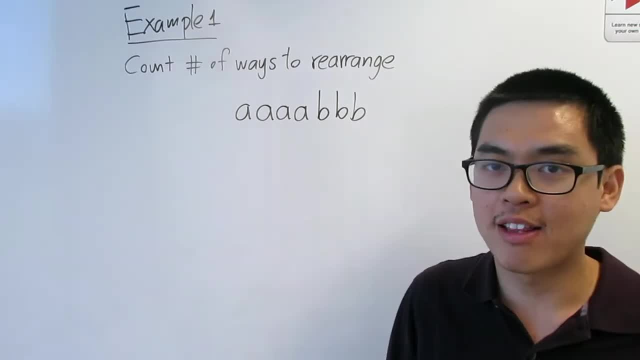 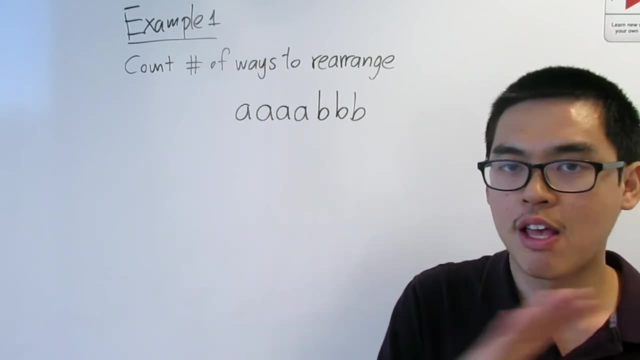 So we have all of the A's and three of the B's at plans. You might be like, oh, we have seen this before you rearrange seven letter, the answer is 7, factorial, Except no, in that case those seven numbers are totally different. this one for A's are the same and these three B's are the same. 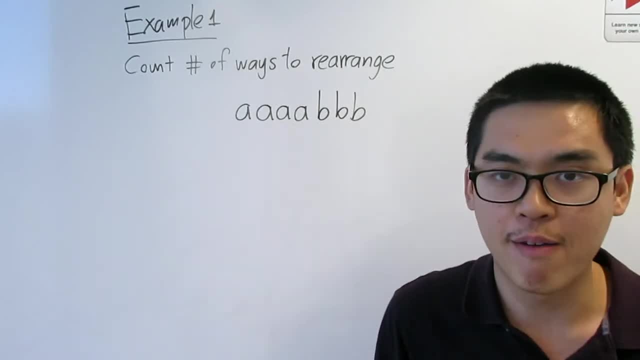 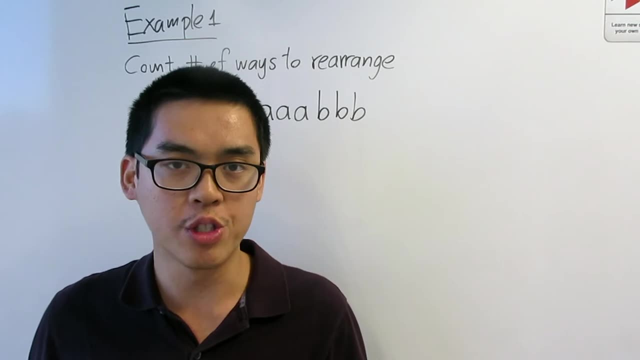 so if we switch up these two A's, you end up with the same configuration because there's no way to Distinguish the first two A's and at first this might not be a problem that you think that you use n, choose k to attack this problem. 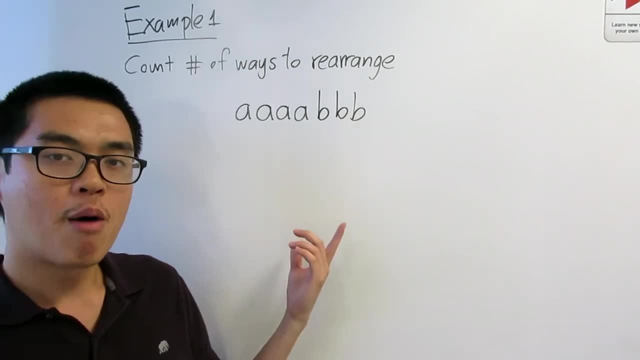 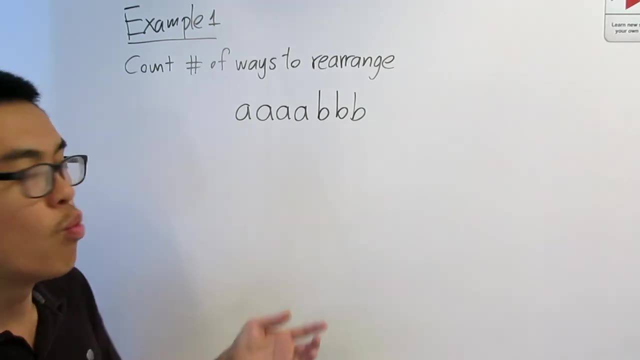 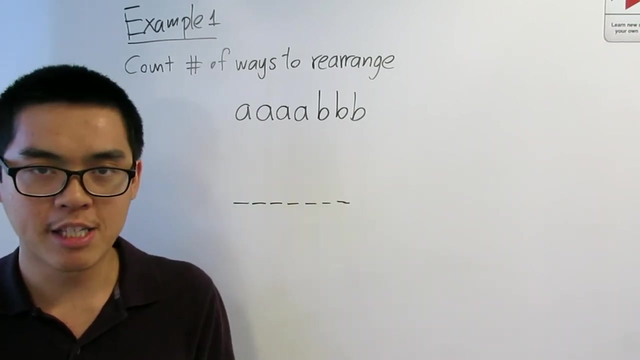 But you can totally do that, And here's how. let's view this problem as follows. So, instead of looking at this number, we look at seven empty spots. Well, why seven? Well, we have seven letters, so we can start with seven empty spots and among these seven, we're gonna choose three of them to place B. 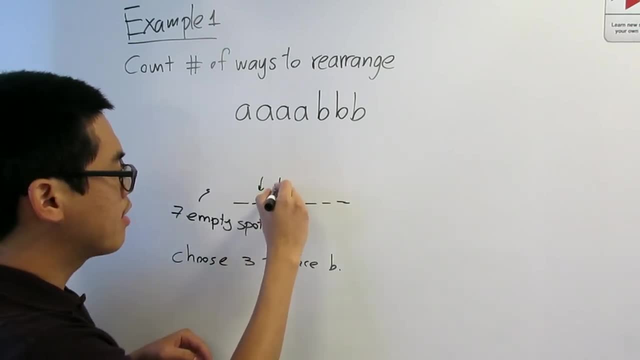 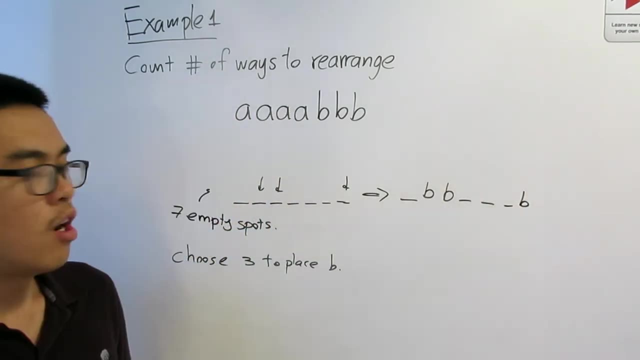 All right. so let's say that we pick This guy, this guy and this guy, so we end up with B, B, three more empty spots and B here. All right. and once we have this configuration A, we just need to go to the rest of the empty spots. 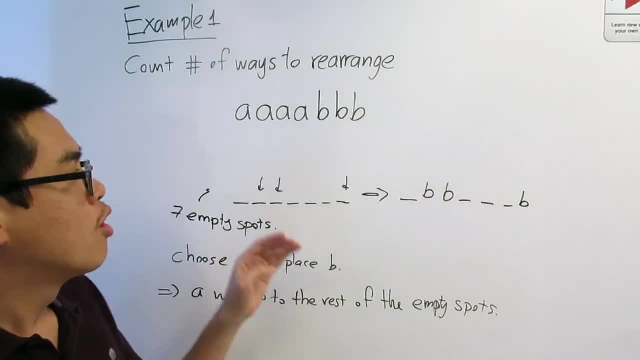 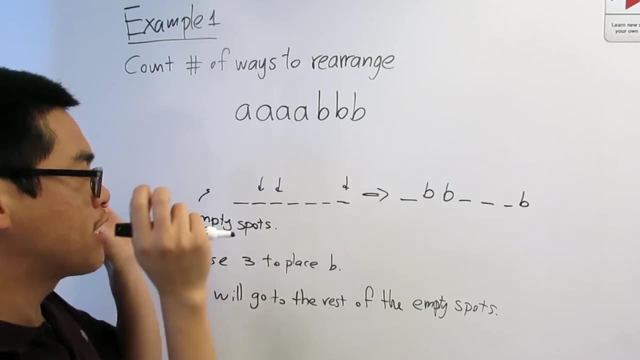 All right. so we kind of like redefine the problem a little bit. So instead of start with these seven letters and we rearrange them, Instead we start with seven empty spots and we place three B's In there and you can imagine that these two operation is kind of like you to the same result. 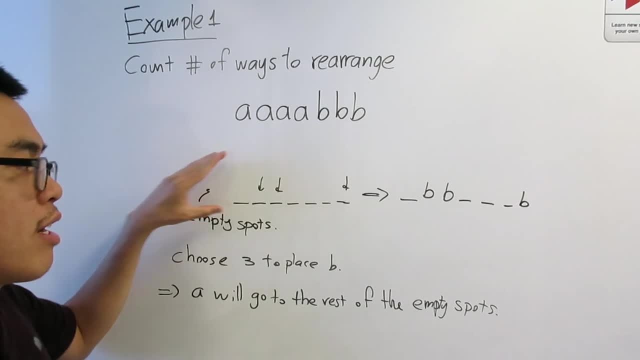 So instead of asking the number of way to do this, we're gonna look at the number of way to do this. But it is precisely this guy right? We just choose three spots. So the number of ways to choose three spots out of seven spots is just seven: choose three. 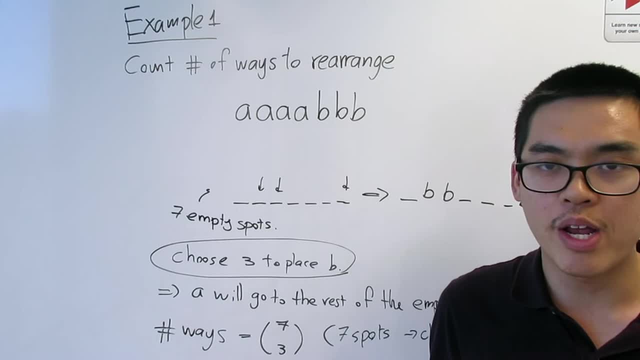 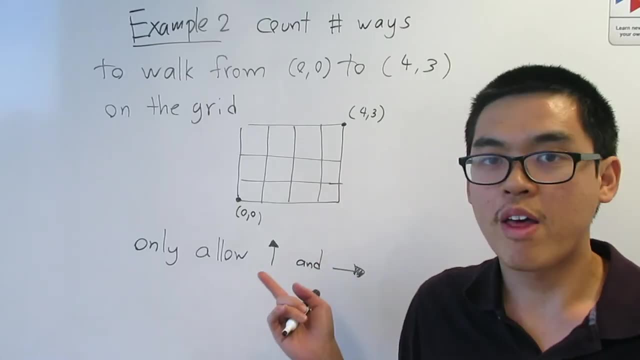 And as we computed twice already, seven choose three is 35, So there are 35 ways to rearrange these seven letters In some way. all right, so let's look at the second example. So let's count number of ways to walk from this point all the way to this point. 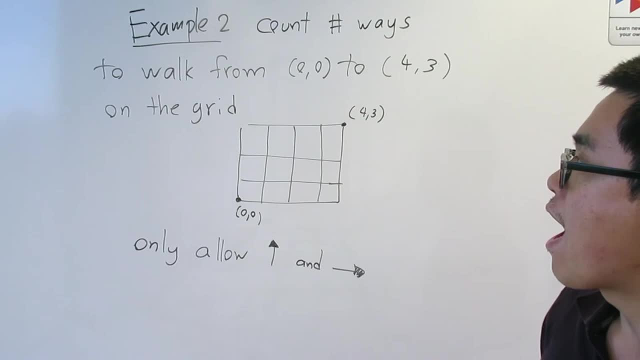 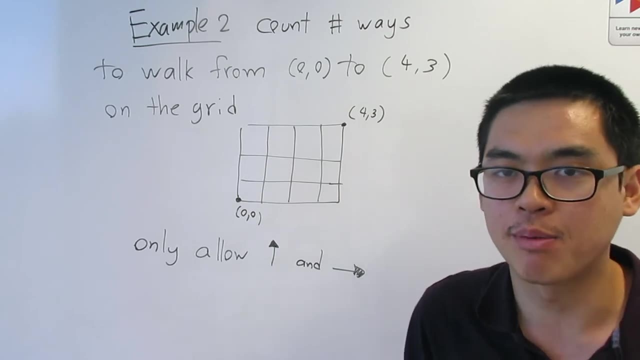 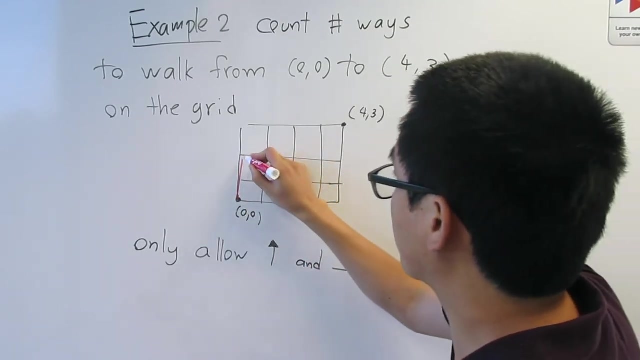 it's point zero, zero. this point is four, three, and You need to walk on the grid and you only allow to walk up and right. So I mean, walk left and now would be just a waste of time, right? so, for example, one way to do is you can go up twice and then you can go right, right, right and 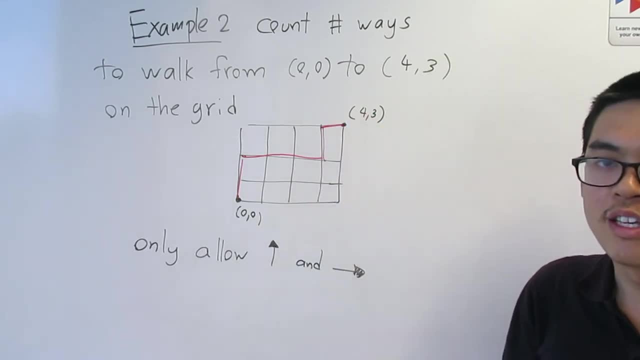 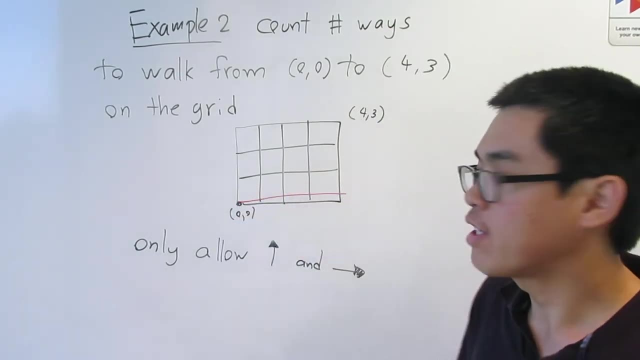 then you go up and then right and then you reach the destination. or if you are a type of person that can only do one thing at a time, then you can Go all the way right first and then go up At the end. or if you are indecisive type of person, you can. 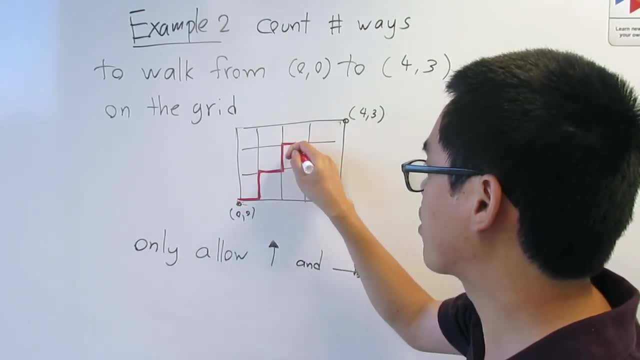 Go right first, and then you go up and then go right and then go up and then go right and then go up and then Go right at the end. All right, so I just show you the three ways you can go from zero. zero to four. three: 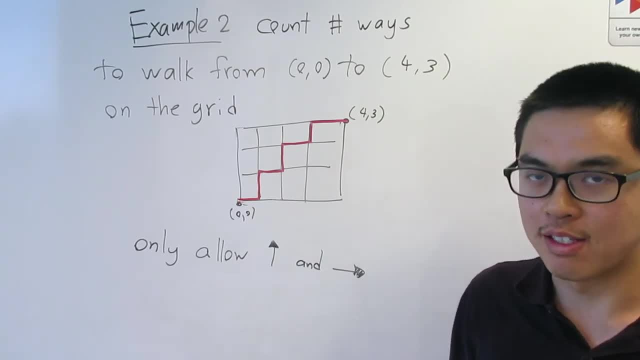 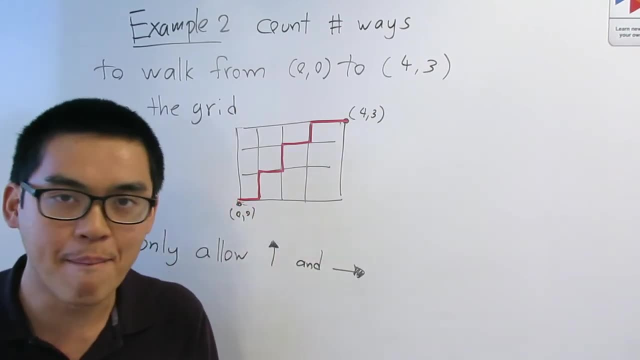 The question is: what is the number of possible ways to do this? And again, this might not seem like a problem that you can use And choose K to attack this problem. right, How do we choose a number of things from a number of things here? 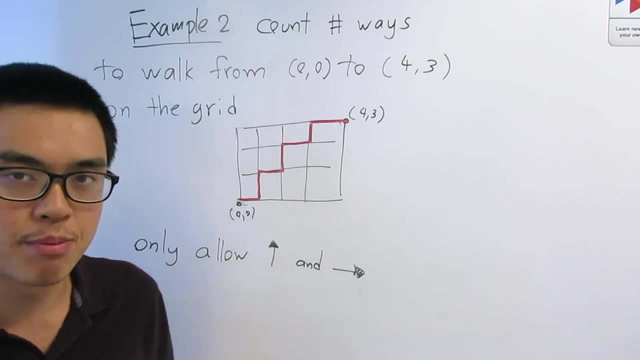 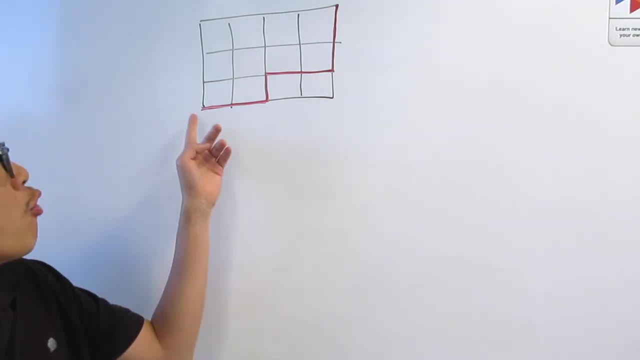 You actually can if you try to look at this problem from different perspective. All right, so let's look at this part as an example. one key observation that you can make is that, no matter how you walk from zero zero to four three, the public consists of four right and 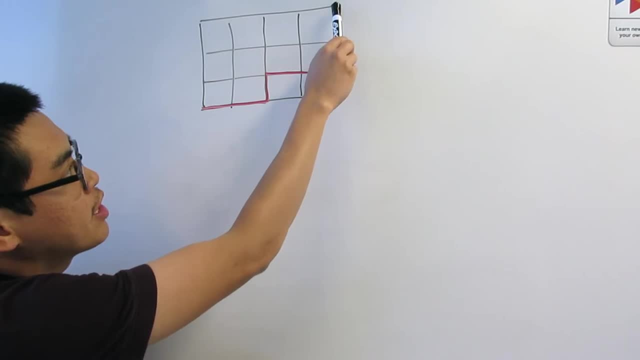 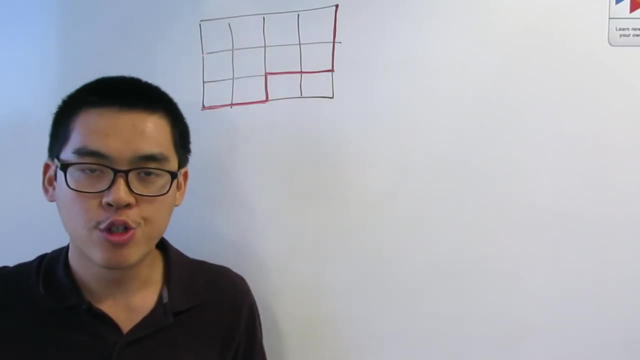 three ups right, because the destination is four step to the right of the original and three step north of the original point. so no matter what you do, You need to do four right at some point and you need to do three up at some point. We can kind of transcribe that into kind of like a sequence of move that we make. 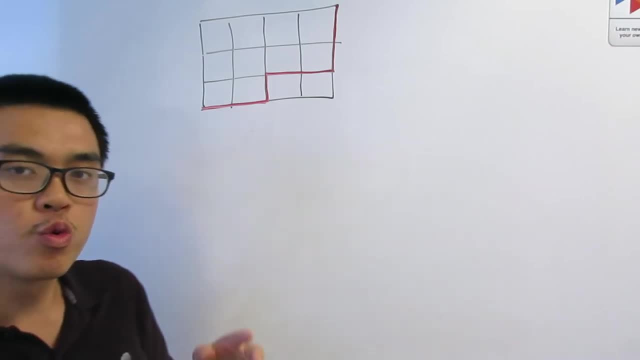 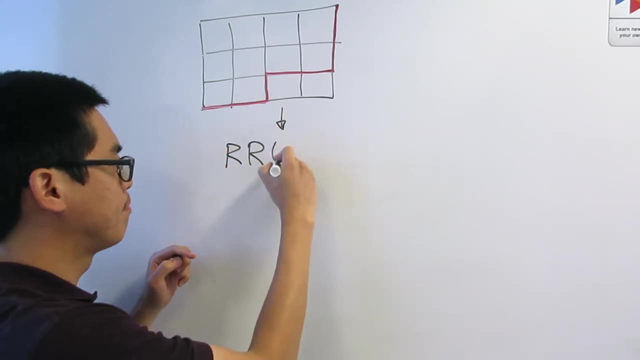 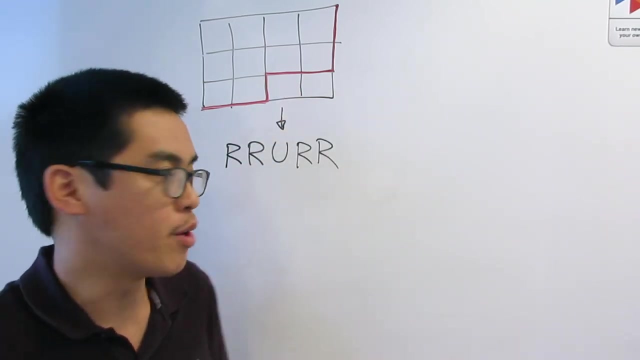 So, for example, this one we do to right bow, So we're gonna denote right by R, So we do Two right and then we do one up Which we're gonna denote by you. then we do two right in a row And then we do two up in a row. 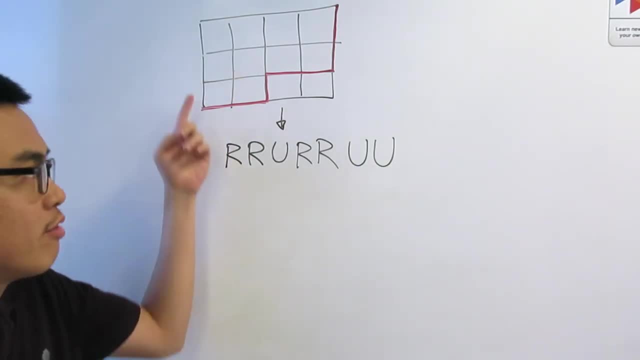 So you can kind of see that you can go back and forth between this right. if Somebody gives you a path from zero, zero to four, three, You can translate to this configuration. on the other hand, If somebody gives you this configuration, you can translate back to this guy to just go to right one up to right to up. 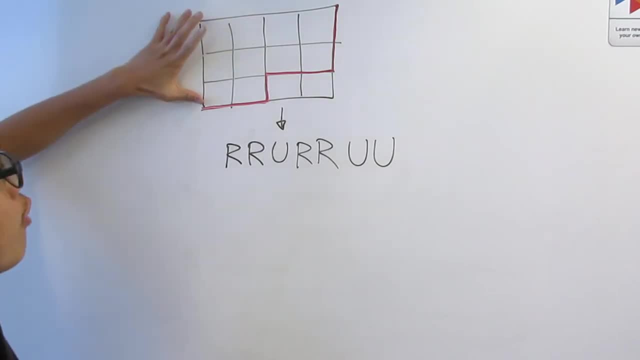 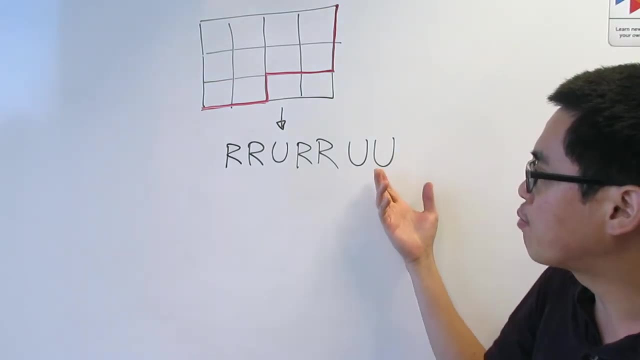 And then you recover this path. So, instead of counting the number of ways to do this, we can count the number of way to do this instead. But what is this? This is simply rearrangement of three use and four hours, Alright. so what's the conclusion? 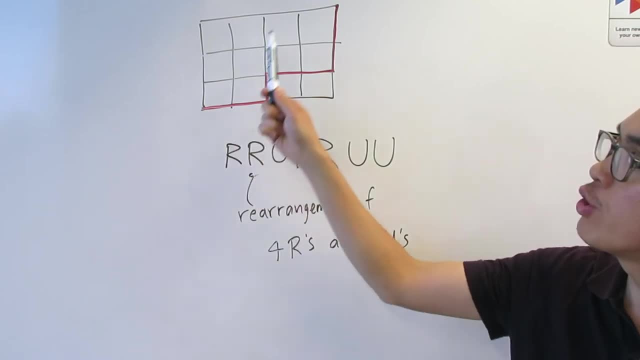 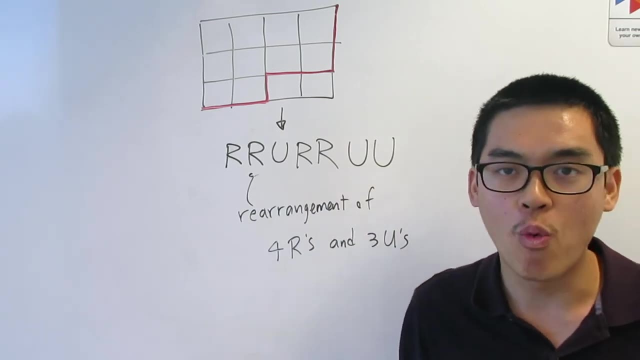 the conclusion is the number of way to walk from zero zero to four. three is the same as number of way to Rearrange for our three. you, in the line which we know from example one that this is simply Seven, choose three right, because there are seven letter. They are three, you. so. 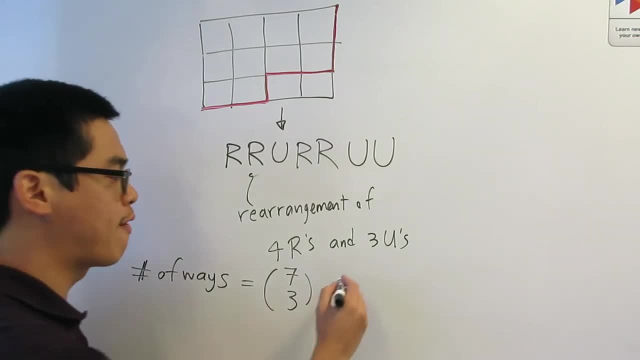 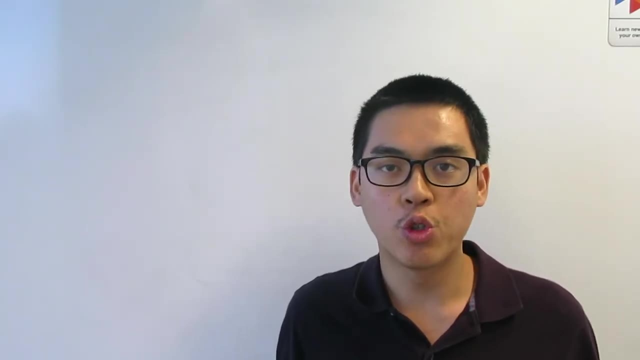 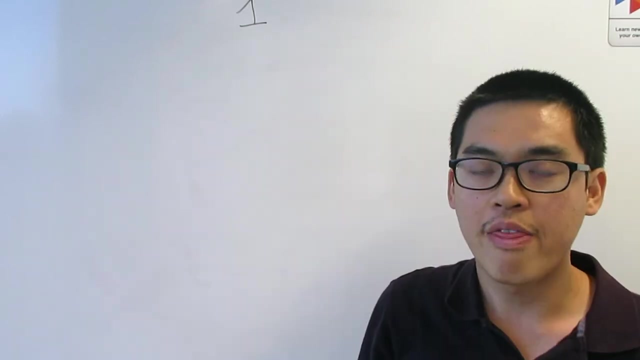 So number of ways? simply seven. choose three, which again is 35. So I want to finish this video with something that directly related to. in choose K, We share the famous Pascal triangle. So here's how it work: you start with one in the first row and the next row, 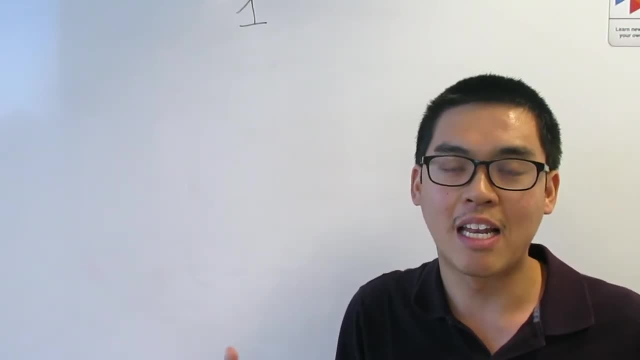 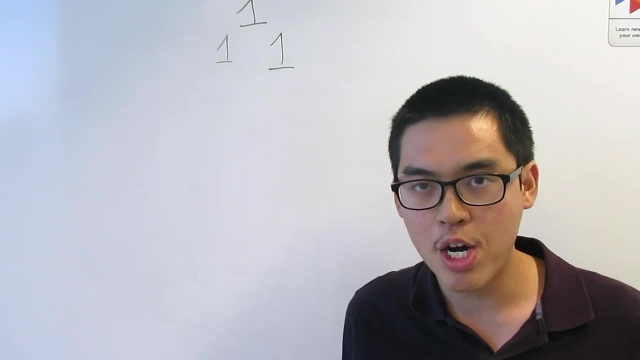 We'll be a pair of one and you kind of place them so that is kind of like form and equilateral triangle. So we have one, one like this and the next you all going to be three numbers and the way we placed them gonna place them So that you have kind of like a triangle that way. 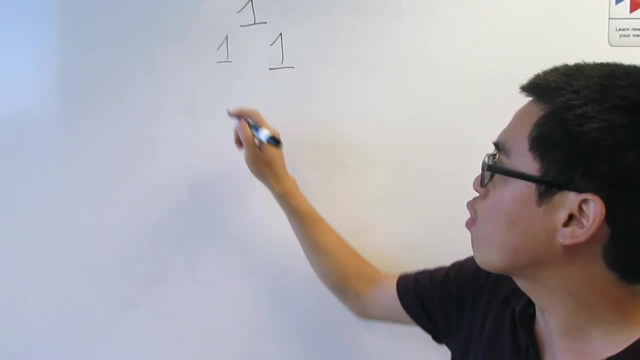 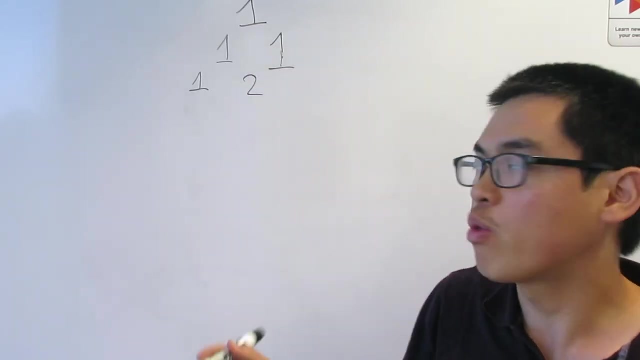 call it a pascal triangle. to determine those number, we start with one at the leftmost number. next number is gonna be the sum of the number that diagonally above it. so this guy gonna be this guy plus this guy, right. so one plus one gonna be two here, and then last guy gonna finish with. 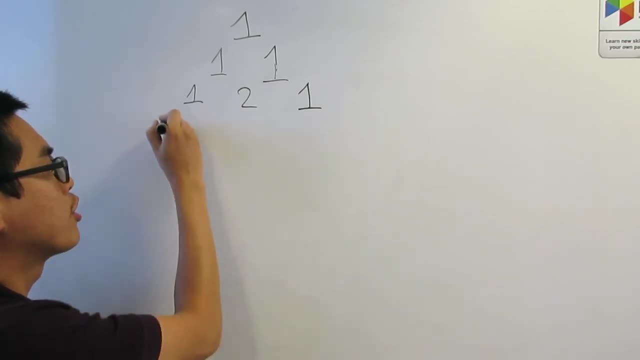 the one again. all right, let's compute the next row together. so it's gonna be one here, because we always start off with the one. this guy gonna be some of these two. so one plus two is gonna be three. this guy's gonna also be three, and this guy gonna be one. this guy gonna be one. four: 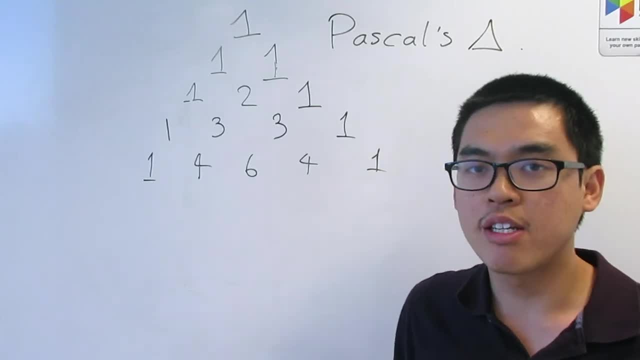 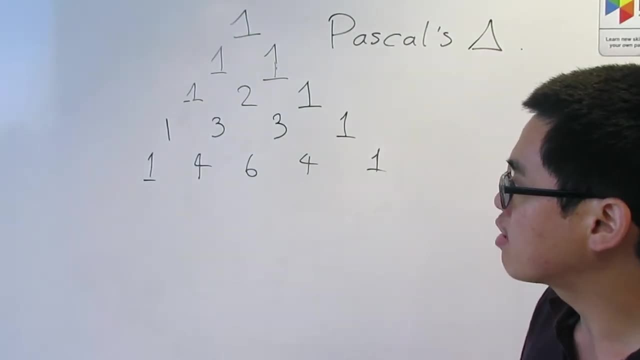 six, four one and, as i mentioned, this is directly related to binomial coefficient, which is in true scale that we talk about. so what is the relationship? so we can try to count the row from the top. so we're gonna call this zero row. we're gonna call this the first row. second, third, fourth. 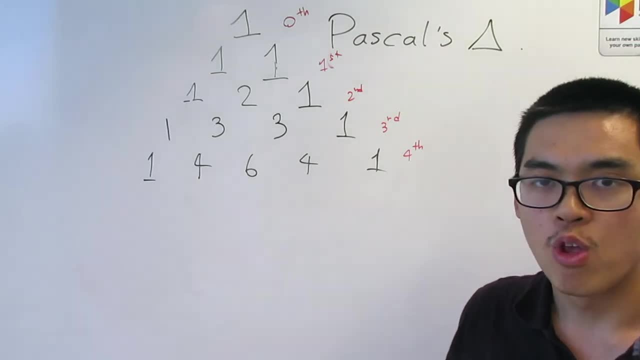 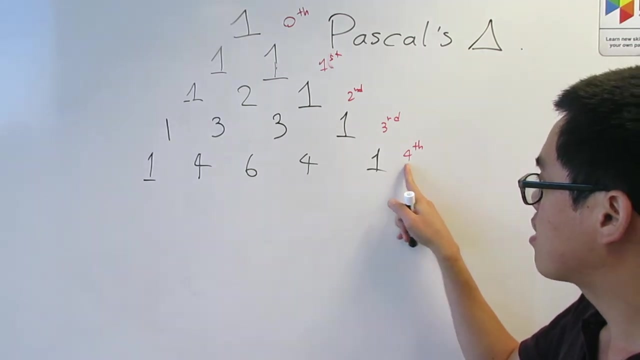 okay. so with this, how does n choose k show up? well, as a matter of fact, all these number will be n choose k, for some n and k, right? how do we determine those n and k? so the row number gonna be n. so, for example, this is the fourth row, right? so all of these will be four choose something. 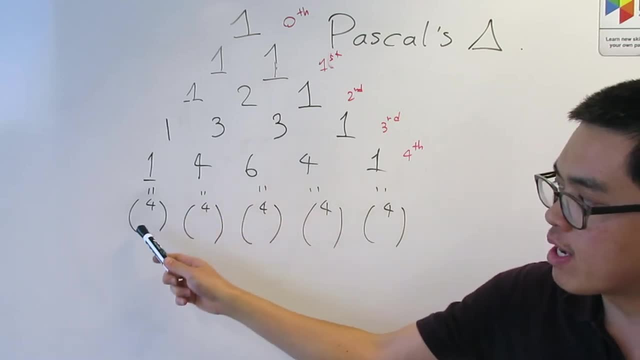 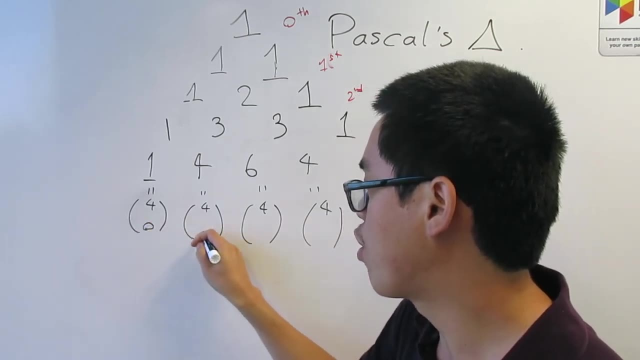 the fourth row will be four, choose something, and those something will be just zero. one, two, all the way to four, from left to right. so the left one is four to zero, four, choose one, four, choose two, four, two, three, four, choose four, and we can go back to the third row. this guy will be three. 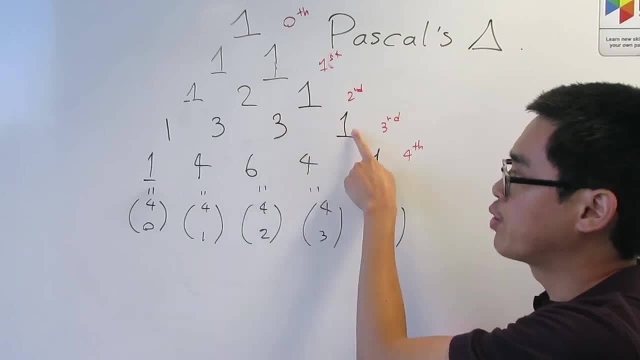 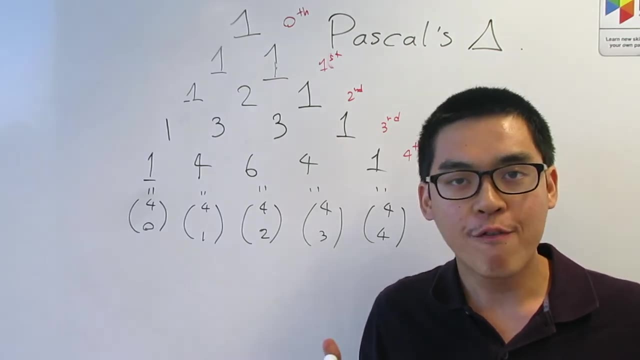 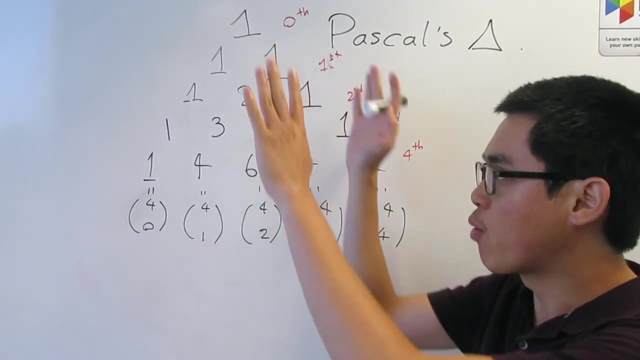 two, zero, three shoes, one, three shoes, two and three, two, three except, for example. so why do we care about pascal triangle? well, it's true that if you want to compute just one and choose k, maybe just like seven, choose three, you don't compute pascal triangle because it's going to be a waste of time.